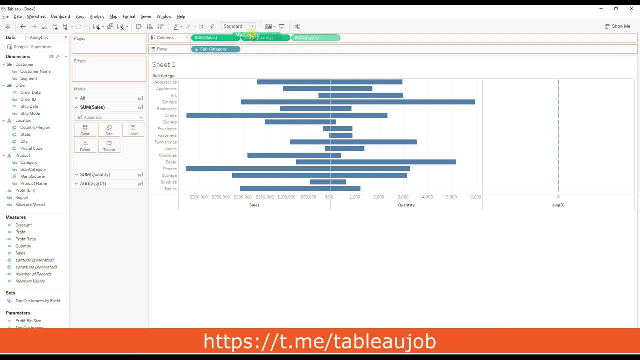 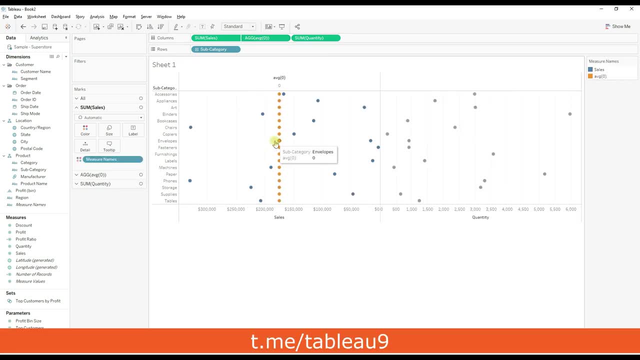 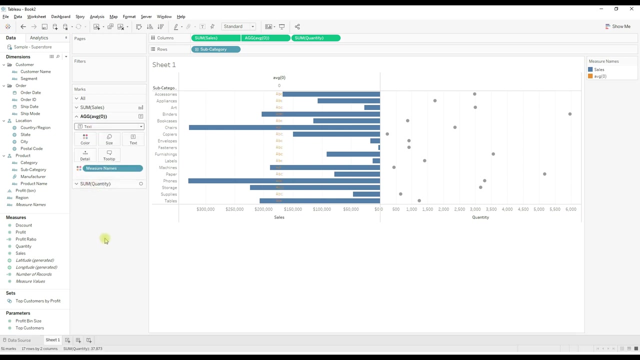 Let me move this calculation next to the sum of sales And now right click and select divert. Now you can see the table axis. So mark type is changed. So you need to go to each mark card and select the required mark type. For sum of sales we need bar and for dummy measure, average zero, we need text. 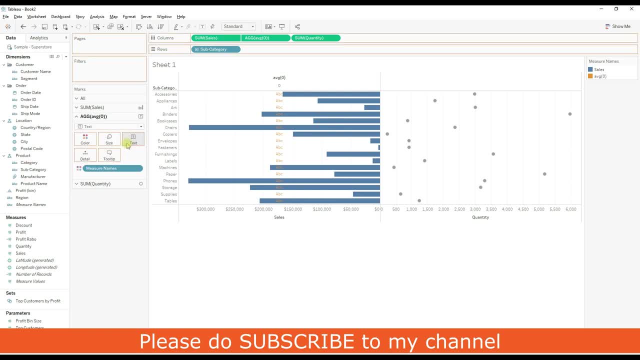 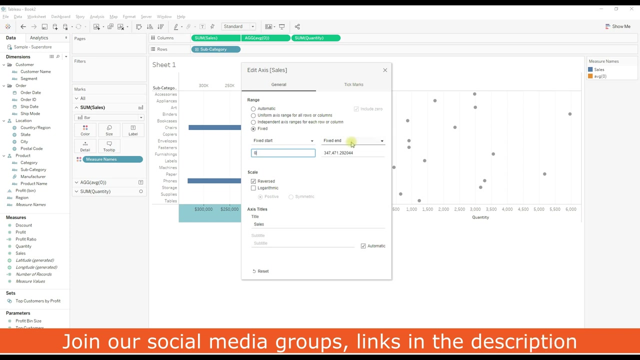 Now drag subcategory onto the text. So we need to synchronize the axis. You can right click and select synchronize axis To remove the space here. you can edit axis and change the range to fixed And the fixed start to zero, Fixed and change it to automatic. 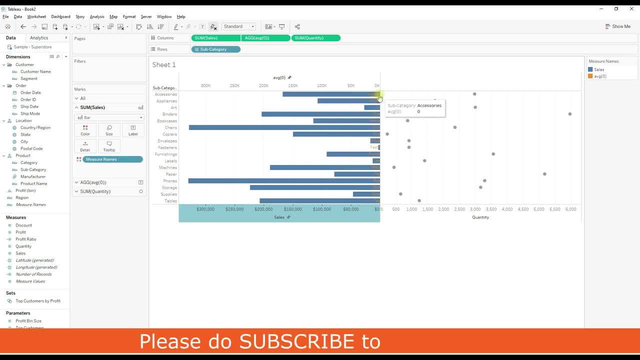 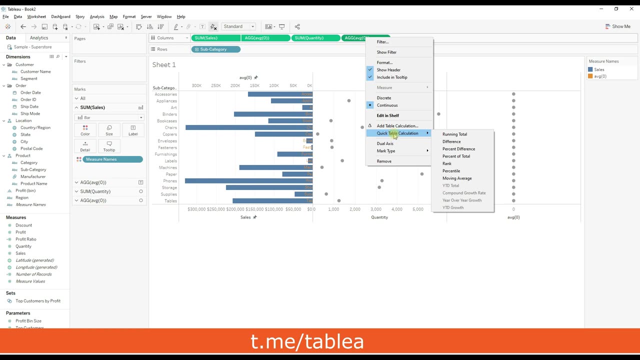 Now the space is removed, So if you see, here we are not seeing the full text, So that's why you need to create another dummy measure: average of zero. Repeat the same steps, Just double click and then select dual axis, So mark type is changed again. 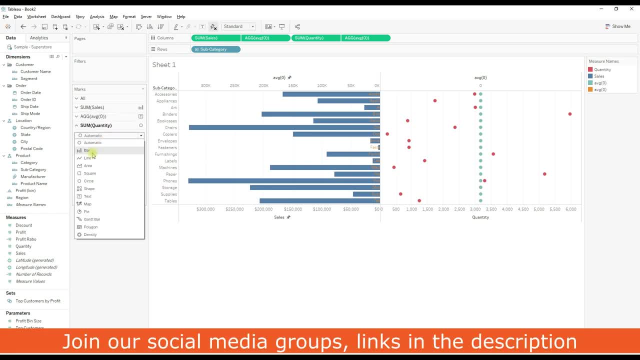 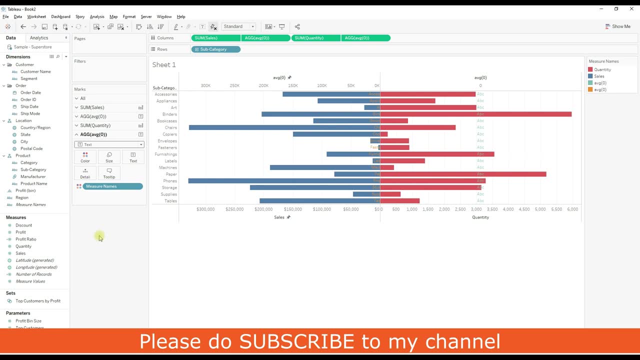 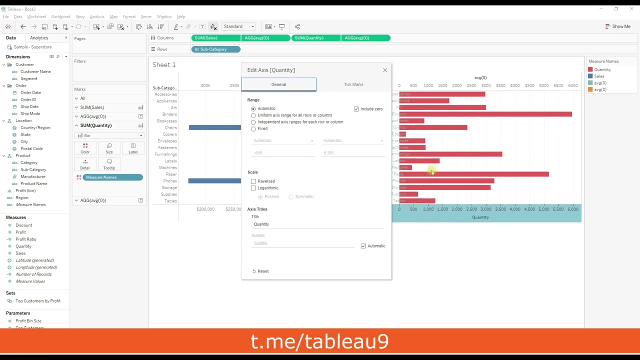 You need to go to the image card and select the desired mark type. In our case it is bar And at average of zero. select text Now drag subcategory to the text. Right click and select synchronize axis To remove this white space. right click edit axis. 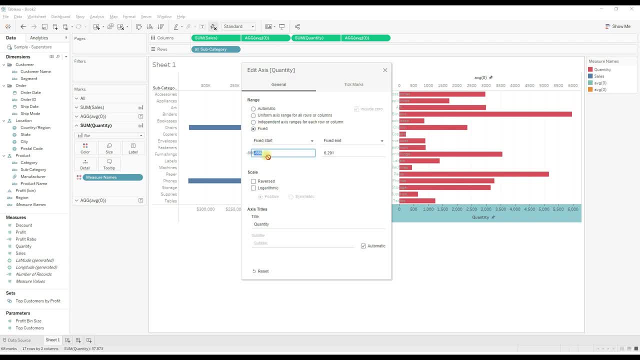 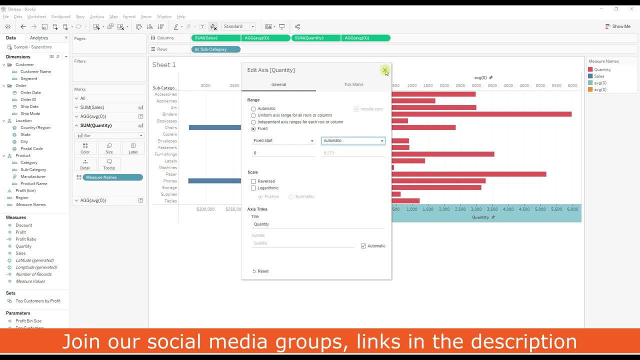 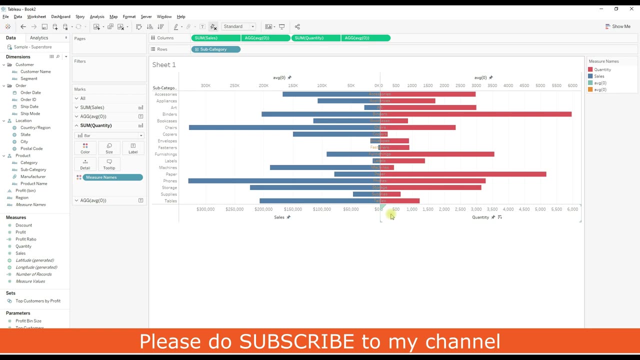 And then choose fixed, Starting from zero. Fixed then to automatic Click close. Okay, now that we have the text showing properly, Full text is visible. now We will do some formatting steps here. First, let me change the Measure colors. Double click to change the colors.